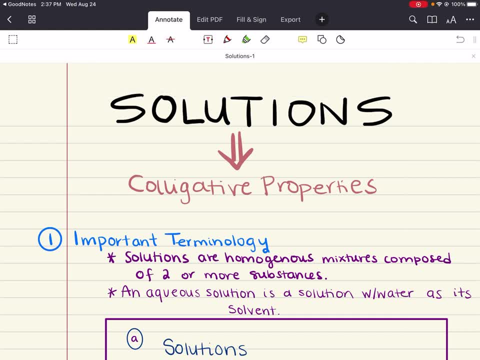 Hello everybody, my name is Iman. Welcome back to my YouTube channel. Today we're going to start chapter 11 for General Chemistry 2.. This chapter is going to cover solutions more in depth. It's going to address two really important questions for us. First, we want to understand what is. 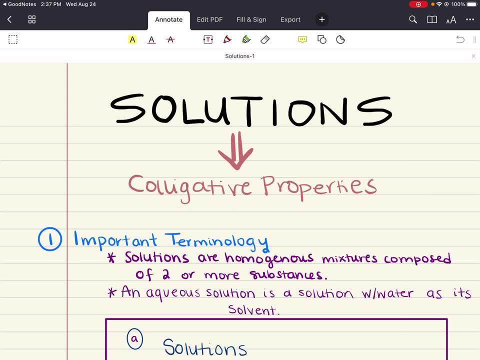 happening at the molecular level in the formation of a solution. In other words, why do some substance dissolve in a given solvent while others do not? And in order to answer this question, we're going to examine things like the solubility rule. We're going to look at intermolecular forces. 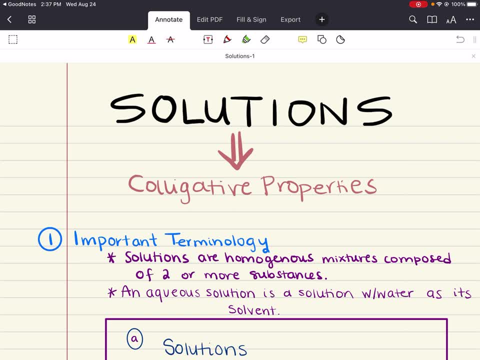 between solvents and solutes and try, with those topics, to reach an answer to why do some substances dissolve in a given solvent while others don't? The second question we want to address and answer is this: What are the properties of solutions? Here we're going to be interested in discussing. 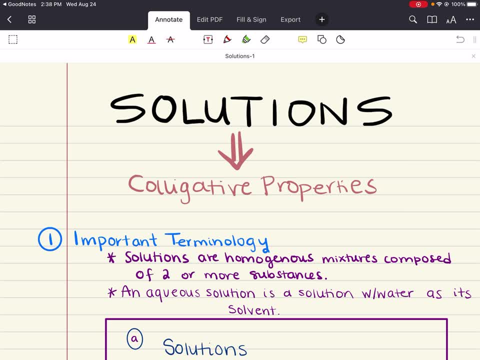 the colligative properties, which are properties of solutions that depend on the concentration of solute particles. So these are going to be the big topics for this chapter that we're going to try to cover. So it's a lot, So let's get started. Let's set the stage for this chapter by defining. 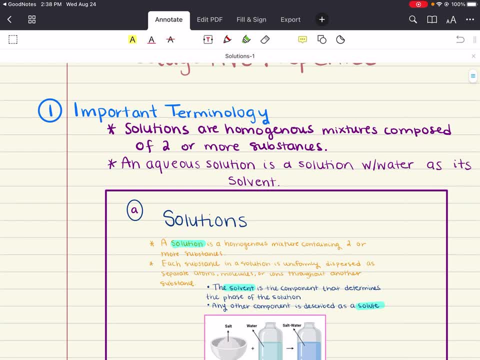 some really important terminology. All right, so we're going to start with terminology One: a solution. What is a solution? A solution is a homogeneous mixture composed of two or more substances. An aqueous solution is a solution with a solution. A solution is a solution with a. 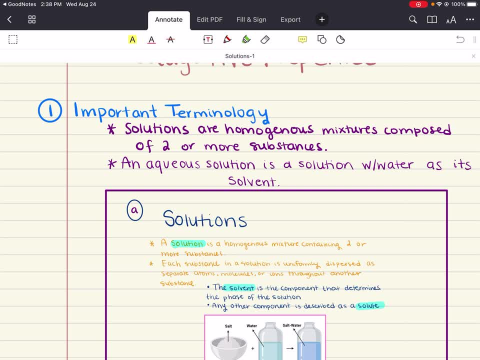 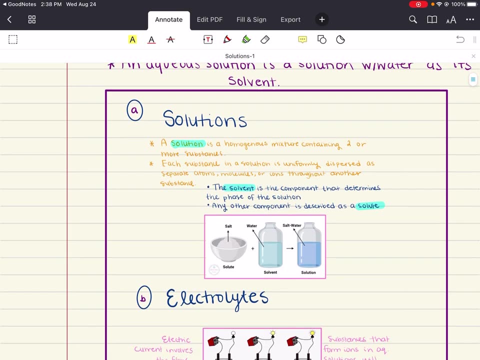 water as its solvent. In order to distinguish between the solvent and the solute, the amount and the original phases have to be considered Now in a two-component solution, if both components were originally in the same phase, the solvent in the greater amount. the solvent is the component. 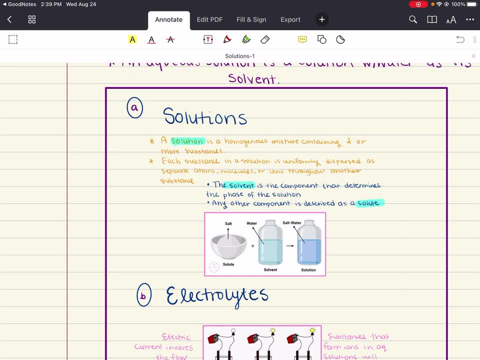 in the greater amount. I'm sorry. All right, so if you have two components in a solution, all right, they're both, Both in the same phase. you're trying to figure out which one is the solvent, which one is the. 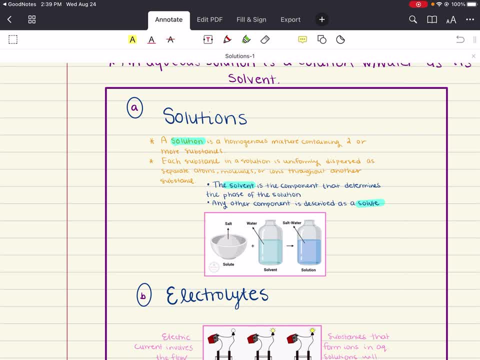 solute. The solvent is the component in the greater amount. If the components were originally in different phases, the solvent is the component that does not change phase. all right at all. not throughout the entirety of mixing the two components, them being in solution. All right. 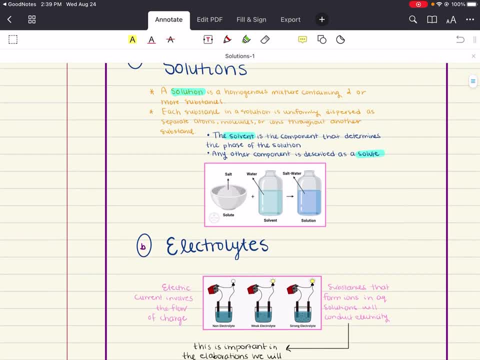 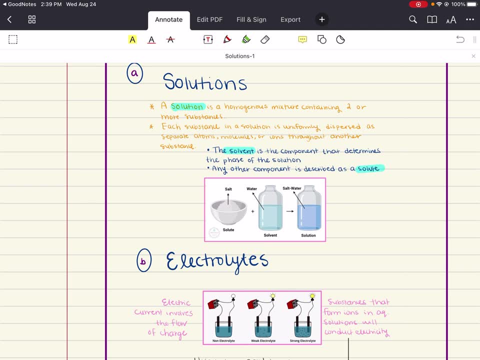 Now, solubility is defined as the amount of solute that will saturate a given amount of solvent at a given temperature. So, with that being said, there are kind of like three really big categories of solubility. all right, You have saturated. 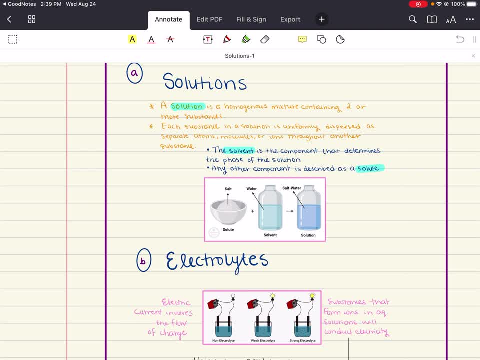 unsaturated and supersaturated. all right. So, once again, what did we define solubility to be? It's defined as the amount of solute that will saturate a given amount of solvent. all right, So we're going to scroll down here where we have this written. 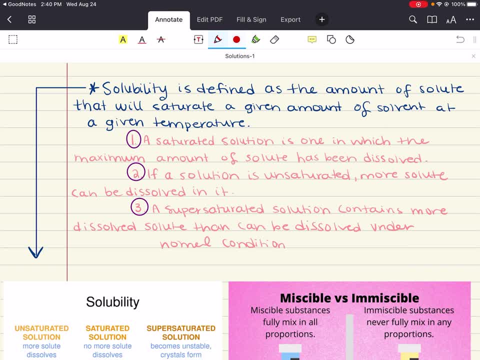 all right. This falls under three categories. You can have a saturated solution, a unsaturated solution and a supersaturated solution. What is each one of these? What is the difference between these three? A saturated solution is one in which the maximum amount of 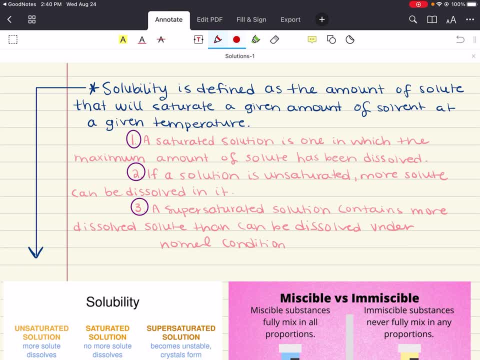 solute has been dissolved. all right, You have dissolved as much solute As you can in the solvent. you have reached that threshold. all right, You have a saturated solution. In a saturated solution, an equilibrium exists between the undissolved solid and the 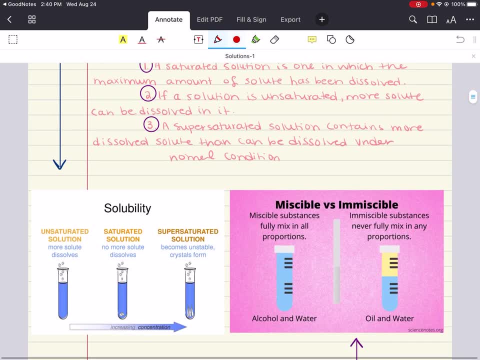 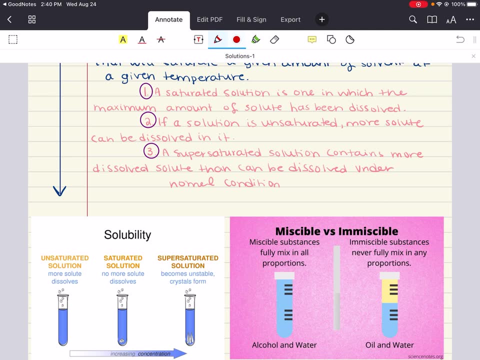 dissolved solute. all right, That is a saturated solution. all right, You have dissolved all the solute you can, possibly with the solvent. all right, Everything else that you might add in terms of solute can no longer be dissolved. No more. solute dissolves because you have a 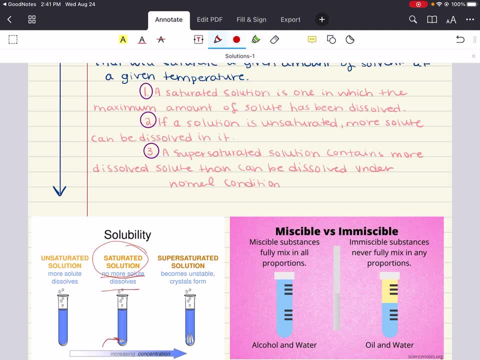 saturated solution. all right, You've reached that threshold. Nothing else will dissolve in the solvent. If a solution is unsaturated, all right, You can keep dissolving solute in it. all right, It has not reached that threshold of: okay, we cannot, we've reached as much solute. 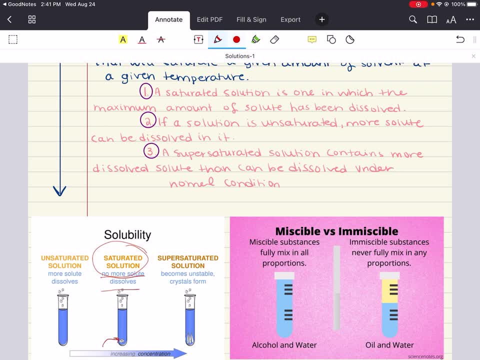 that we can dissolve in the solvent Unsaturated, have not reached that threshold anymore, any yet, and so you can add more solute and it will dissolve, because the solution is unsaturated. A supersaturated solution is a metastable state, meaning that, although it is temporarily stable, any slight disturbance will cause precipitation. 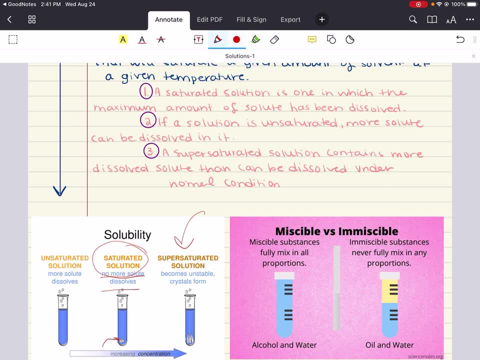 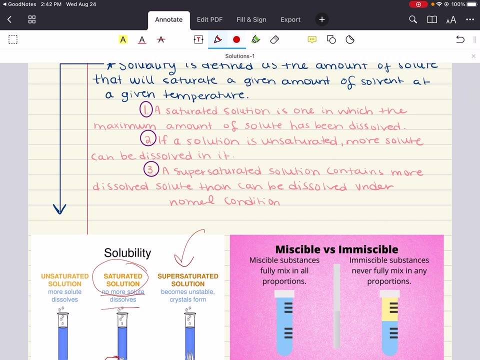 to occur, all right, And that's going to result in the more stable saturated state. all right, Those are three important categories that fall under the conversation of solubility. all right, You have saturated, unsaturated and supersaturated. Now electrolytes. 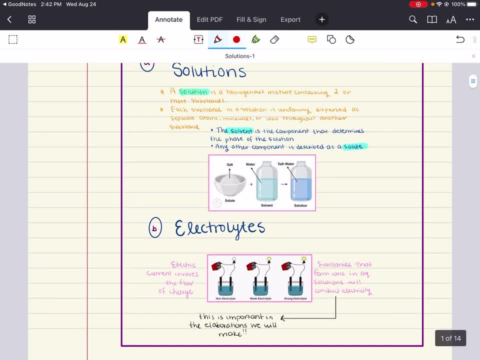 we have covered this before in General Chemistry 1, but these are terminology that are important to be able to understand when used in conversations, when used in discussions about chemistry. so I want to just redefine electrolytes. Electrolytes are substances that form. 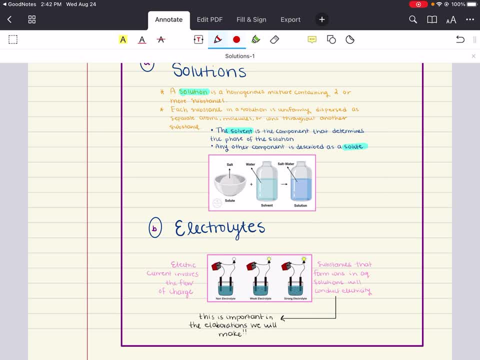 on the surface of the body and they are used to form on the surface of the body. So if you put an electrolyte in solution, it will dissolve and it will form ions. Take, for example, table salt, sodium chloride. If you put sodium chloride in water, all right, sodium chloride is. 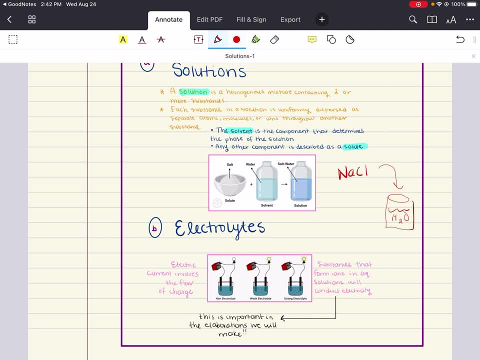 going to dissolve in water and it's going to form ions. It will dissolve and it will form sodium plus ions and chloride minus ions, all right. So if you put an electrolyte in solution, it will dissolve and it will form ions. So electrolytes are substances that form ions when dissolved in. 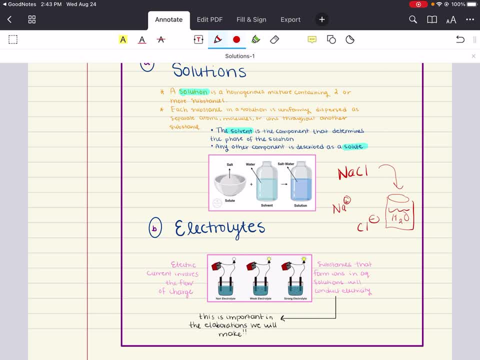 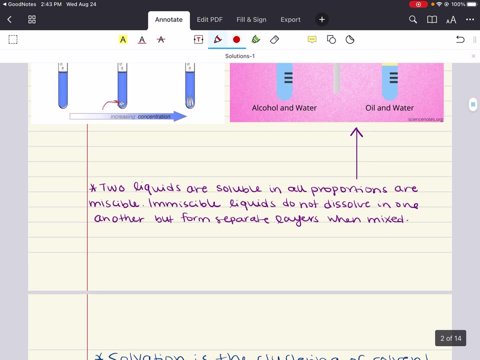 aqueous solution. Non-electrolytes, on the other hand, are actually substances that are soluble in water, but they do not dissociate into their ions in aqueous solution, so they will stay whole, all right. Now, in addition, some more important terminology: two liquids that are soluble: 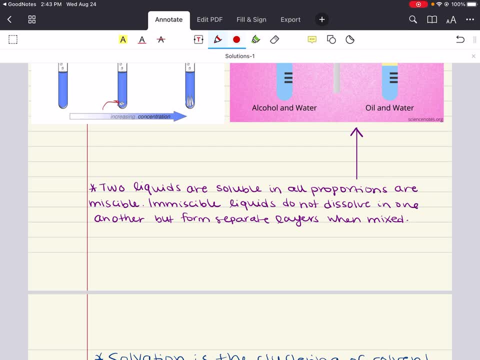 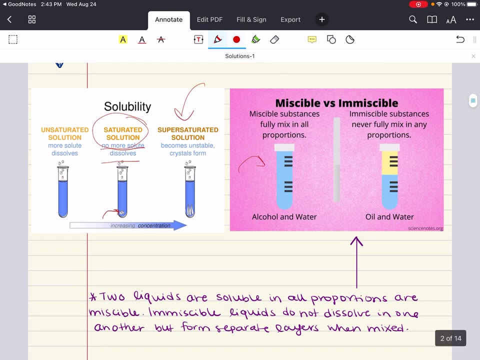 in all proportions, are termed miscible liquids. All right, Inmissible liquids are ones that are not going to dissolve in one another. Instead, they're going to form separate layers when they're mixed together. all right, Good examples: all right, Alcohol and water. if you mix those together. all right, they are soluble in all. 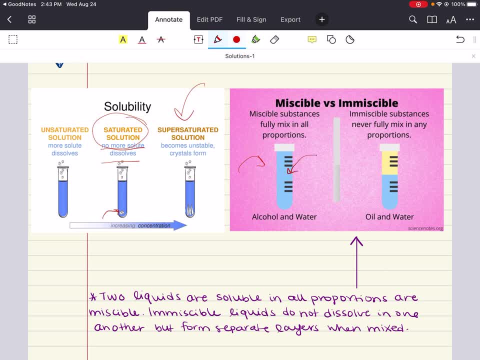 proportions. You actually will look at alcohol mixed with water. You cannot tell where the alcohol starts and ends or where the water starts and ends. They are mixed in, They are dissolved in each other, all right. Inmissible liquids do not dissolve in one another. Things like oil and 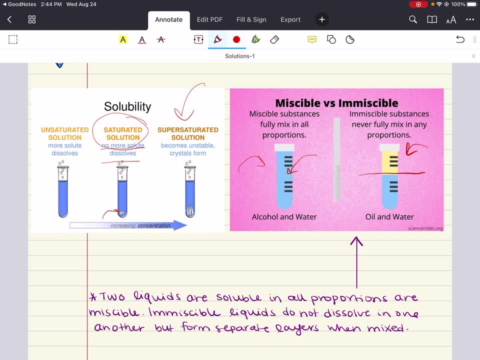 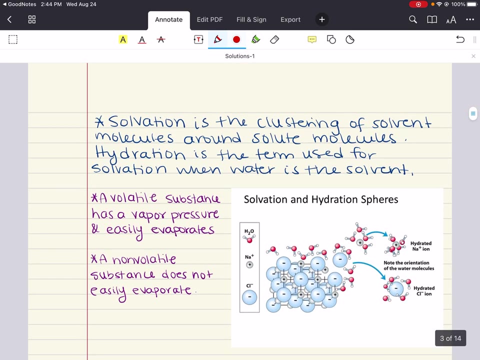 water are going to separate, all right, And you can distinguish the oil phase from the water phase. They're not going to mix, They're not going to dissolve in one another, all right. So that's the difference between miscible and immiscible. Now solvation is another very important term. 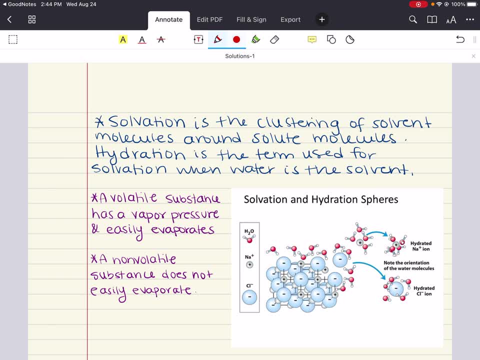 all right. Solvation is the clustering of solvent molecules around your liquid. So if you mix two solvents together, you're going to have two solvents around your solute, all right. So one more time, solvation is going to be the clustering- all right- of solvent molecules around a solute. 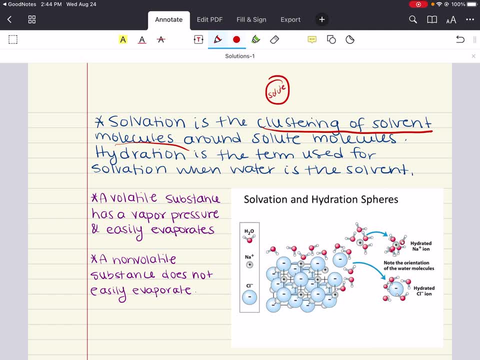 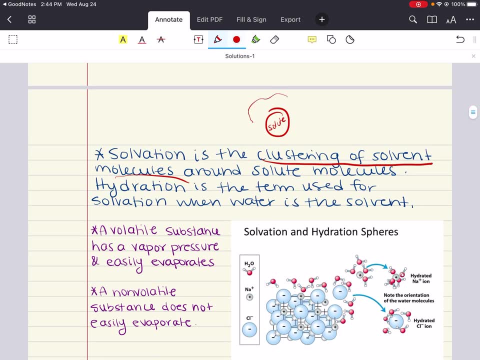 molecule. So you have your solute, all right, You have your solute and it is going to be clustering around. it is going to be your solvent molecule. So you might have several solvent molecules, all right, that are going to cluster around your solute molecules, all right, So 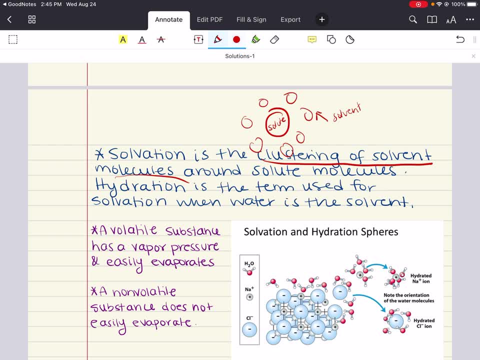 remember, if you mix two solvents together, you're going to have two solvents around your solute molecule. Again, always, reiteration is important. A solution is a homogeneous mixture, all right. An aqueous solution is a solution with water as its solvent. In a two-component solution we generally speak. 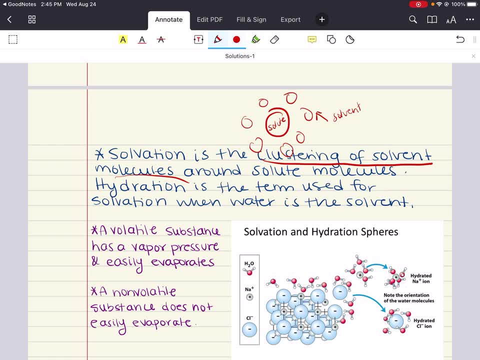 of the solvent and the solute. all right Here, when we talk about solvation, we're talking about the clustering of those solvent molecules in your solution around your solute particles. Now under solvation is another category term: hydration. Hydration is the term used for solvation when the solvent 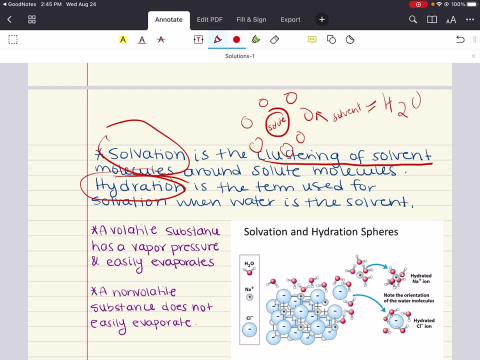 is actually just water all right. So if your solvent is water, all right, you call this process hydration all right. where your solute is surrounded by water, it's called hydration all right And as a general broad category, all right. we can say solvation. Solvation is the 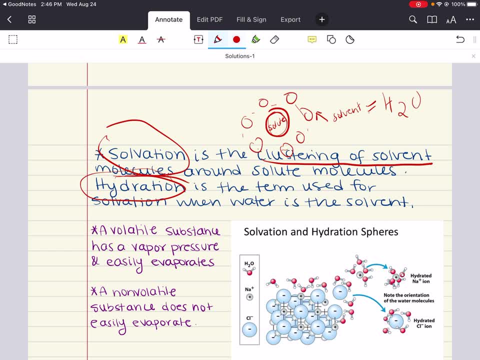 clustering of any solvent, not just water, but of any solvent. So if your solvent is water, any solvent around your solute molecules all right. And last but not least, two more terms- we covered these last chapter: volatile and non-volatile, but again important to reiterate. 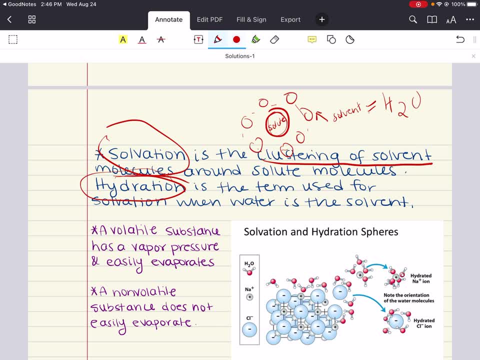 and why not? right? Because we're in the learning process. hearing things being repeated is the best way to learn them. A volatile substance has a vapor pressure and it will easily evaporate, as opposed to a non-volatile substance That is not going to easily evaporate. all right, So those are all the important terminology that 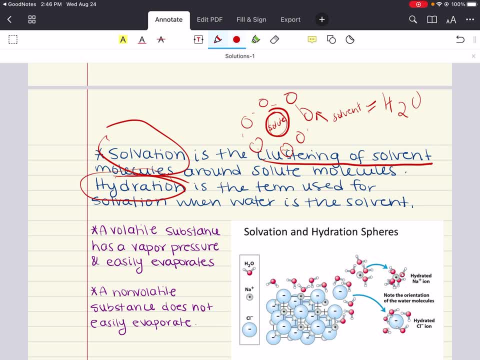 we're going to need to understand in order to have a conversation about solutions, the solution process and colligative properties. So hopefully that was a good review of all these terms that we have used and learned, especially in general chemistry one. Now we're going to apply them. 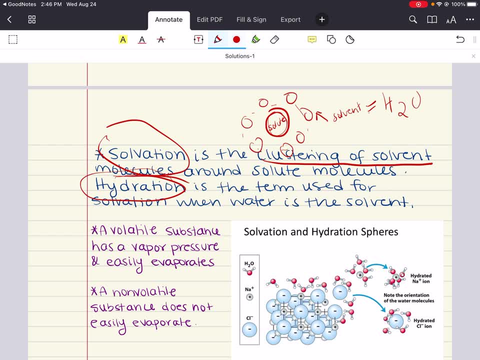 to a different topic that we have not covered, about solutions right. So now, with all this proper understanding, we're going to have a conversation about solutions and we're going to discuss the solution process. all right, Here we're going to ask an important question. 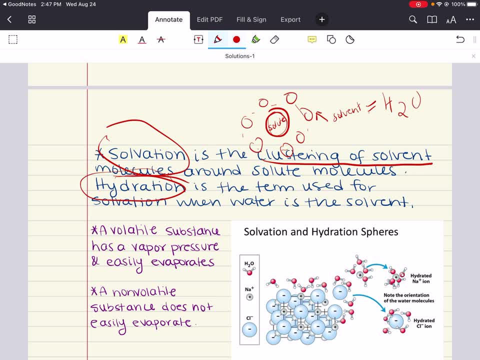 What is the driving force of solutions? all right. In other words, why are some substances soluble in a particular solvent, while others just aren't? all right, What is this driving force? Chemists often refer to this rule. that kind of explains this problem. all right, This question that we're 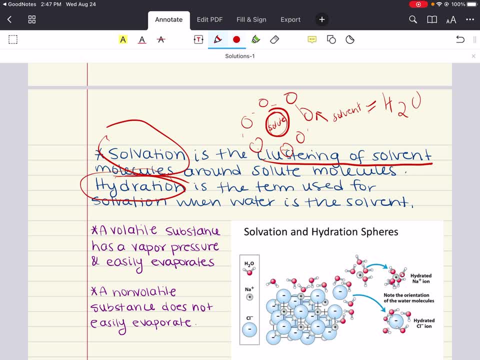 asking Chemists will often refer to this rule. that kind of explains this problem. all right, This will refer to what is called the solubility rule, and you might have heard it before. Like dissolves, like This is a short, simple way of saying that nonpolar solvents are going to dissolve nonpolar 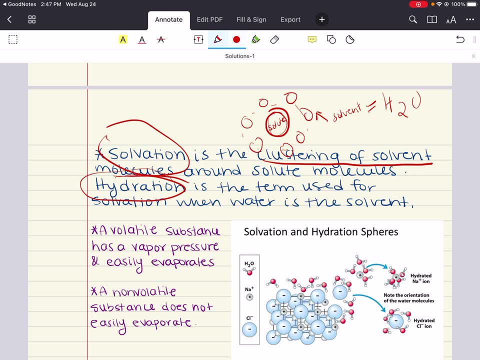 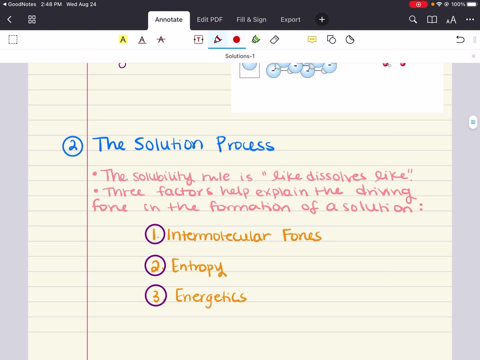 solutes. Polar solvents are going to dissolve polar and ionic solutes, And so, then, to understand the driving force in the formation of a solution, we're going to have to discuss three important factors: entropy, intermolecular forces and the energetics of the solution process. These three 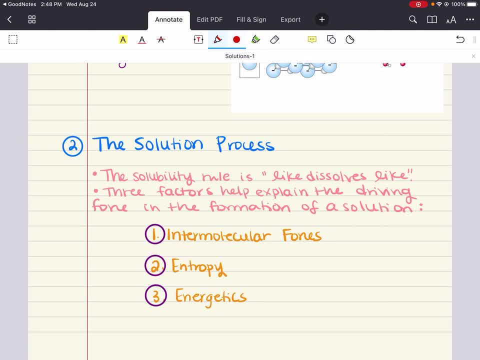 topics, along with our solubility rule of like dissolves like, is going to give us a full understanding of what the driving force of solutions is. Okay, so, like dissolves like, let me repeat, is a short, simple way of saying: nonpolar solvents dissolve nonpolar solutes. 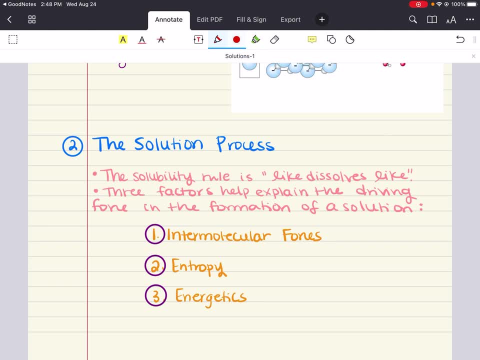 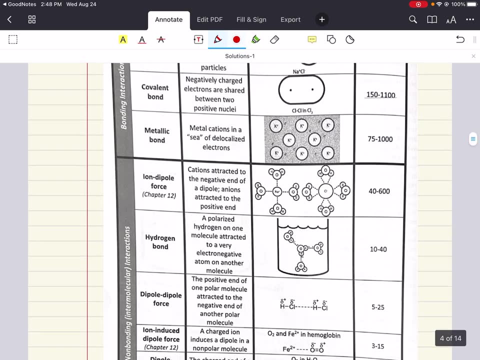 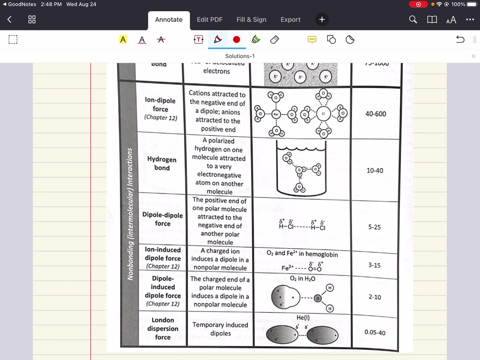 Nonpolar solvents dissolve polar solutes. All right, like dissolves, like. Now let's understand the driving force and let's start off with our intermolecular forces. Here's the table of all our intermolecular forces. There are six of them. All right, we covered three last time. We're still. 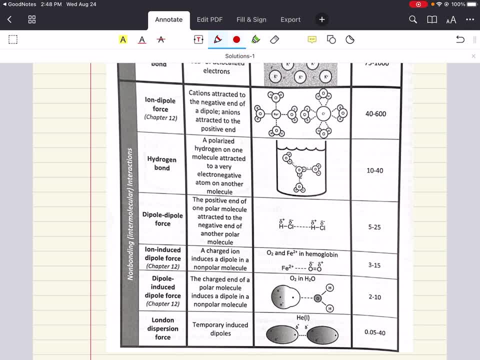 going to review them again, All right. and then we're going to introduce three more that we have not covered yet, that we're going to cover in this chapter, All right. so for intermolecular forces, there are six types that are going to exist between solute and solvent. All right, 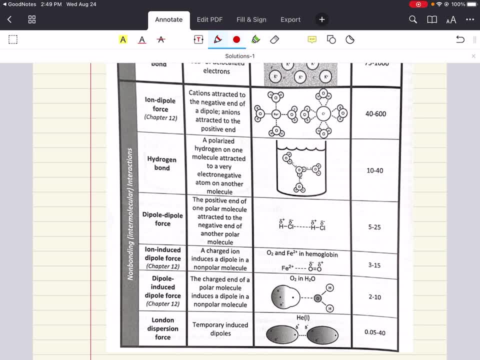 the first three that we're going to talk about. we covered last chapter. we're going to recover today. First one is dipole-dipole forces. All right, that's this one right here. All right, dipole-dipole forces. We learned that a polar molecule is one that has an unequal distribution. 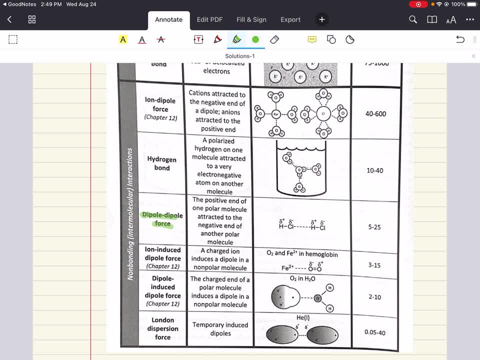 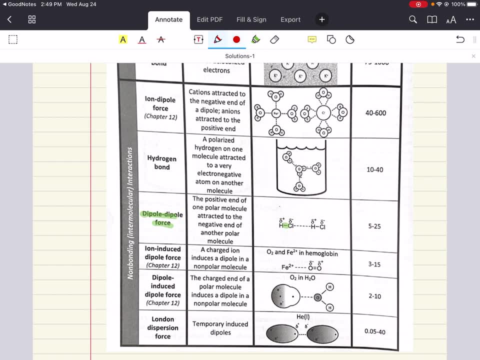 of charge, All right. polar covalent bonds: they're going to share electrons to form a bond. Sorry, not right there. right here, That's a polar covalent bond, right there between the hydrogen and chloride. They're sharing electrons with each other, but unequally The. 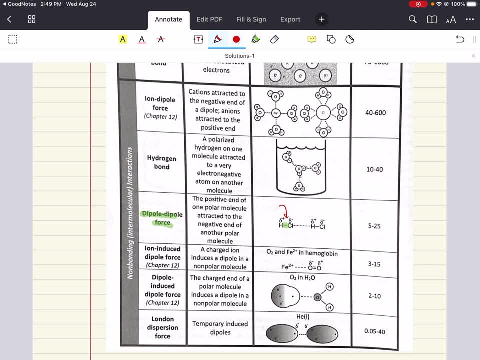 chlorine likes the electrons a little more than the hydrogen does, so it pulls them a little towards the chlorine. All right, and what you get are these partial charges. partial negative on the chlorine because it likes to hog the electrons a little more on its side and leave the hydrogen a. 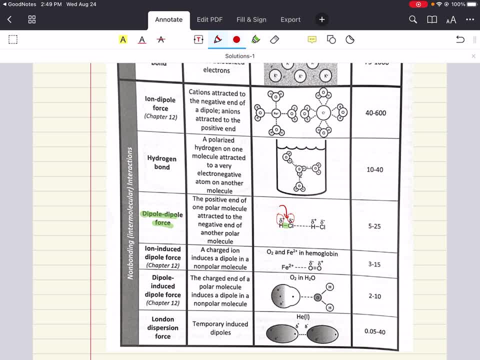 little empty in electron density, and so the hydrogen has a partial positive. All right, so we learned that polar molecule is one with an unequal distribution of charge resulting from the shape and the nature of the bond. All right, now, when you place a polar, 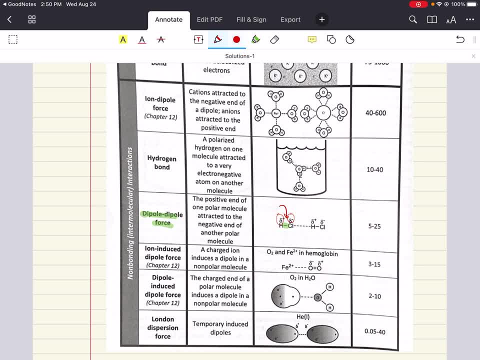 molecule in a magnetic field, it's going to behave as if it has a center of positive charge and a center of negative charge. hence these partial negative, partial positive charges. And, in other words, what we can say is that this hydrogen, bonded to a chlorine, it possesses a positive 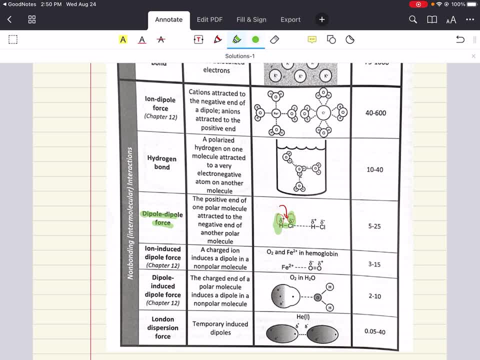 dipole, All right, where the partial positive on one it possesses a permanent dipole. It has these partial positive, partial negative regions And what happens with this is that the partial negative- let me circle this in blue- the partial negative of one molecule is going to interact. 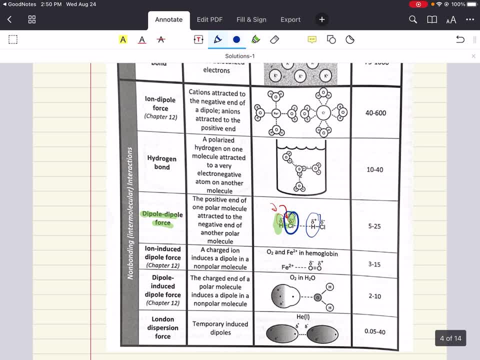 with the partial positive of another- hydrochloric. All right, so we have the partial negative of one HCl molecule interacting with the partial positive of another HCl molecule. This dipole-dipole force exists between polar molecules such as hydrogen chloride. All right, what you see here, this interaction between the partial negative of one. 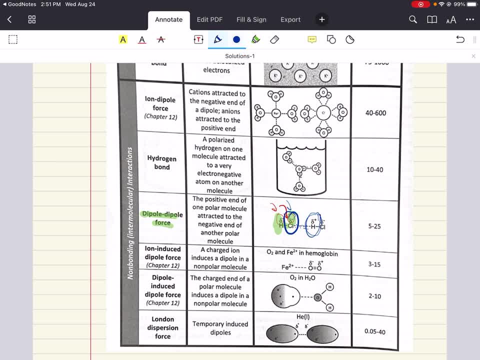 hydrogen chloride and the partial negative of another hydrogen chloride. we call this a dipole-dipole force: The positive end of one polar molecule is attracted to the negative end of another polar molecule. Fantastic, Hydrogen bonding is another thing we covered last chapter. that's very important. All right, a hydrogen bond is going to be this intermolecular. 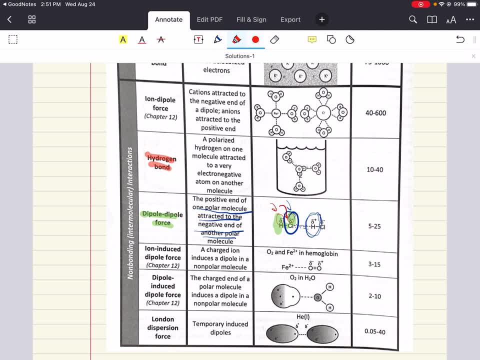 attraction between a polarized hydrogen on one molecule and a very electronegative atom on another. All right, so this is going to really occur between hydrogen atoms on one molecule with a very electronegative atom on another. What kind of very electronegative atoms are we talking about? 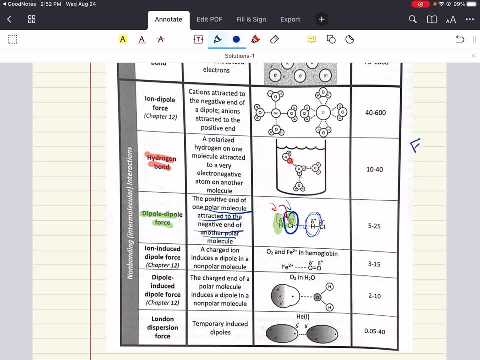 There's three big ones. All right. hydrogen of one molecule might interact with a fluorine atom of another molecule, or an oxygen atom of another molecule, or a nitrogen atom in another molecule- All right. so when a molecule contains a hydrogen atom that's covalently bonded or attached to, 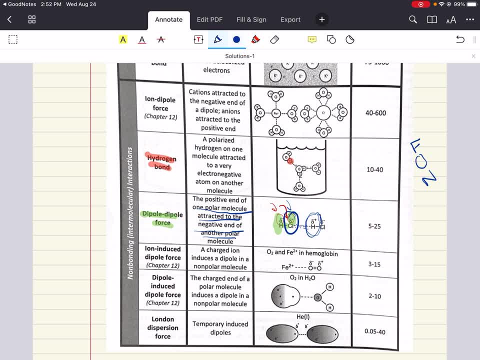 fluorine, oxygen or nitrogen, there's going to be a large difference in electronegativity. All right, that's going to make the bond polarized, where the hydrogen is going to have that partial positive charge And that partial positive charge associated with that hydrogen might interact. 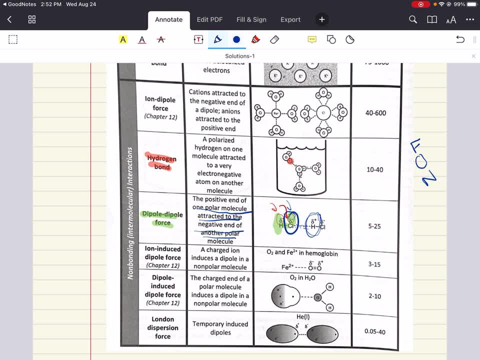 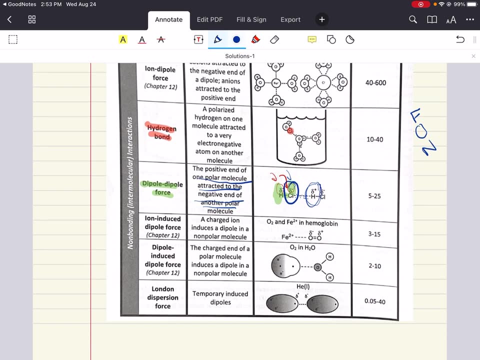 with another very electronegative atom like fluorine, oxygen or nitrogen on another molecule, All right. notice how all these intermolecular interactions are between atoms of one molecule to another molecule, All right, whereas chemical bonds were atoms within the same molecule forming. 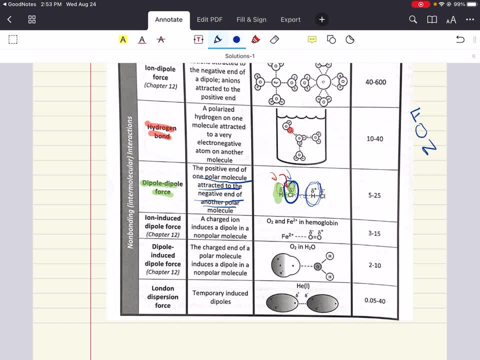 bonds. All right, that's the difference that you need to make sure you are clear on, All right, so as not to confuse this. All right, so hydrogen bond- a hydrogen of one molecule- is going to interact with, say, an oxygen atom of another molecule, And it's going to interact with, say, 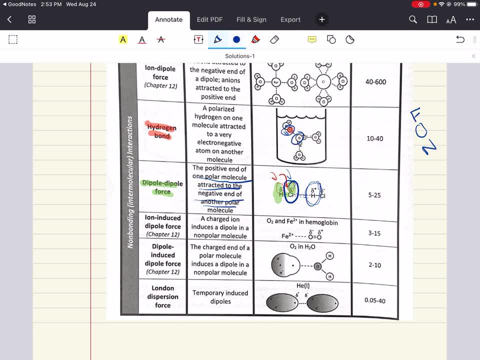 this intermolecular interaction. This one specifically, is called a hydrogen bond. All right, a polarized hydrogen on one molecule is attracted to a very electronegative atom on another molecule. Fantastic London dispersion forces. This was also one that we covered last. 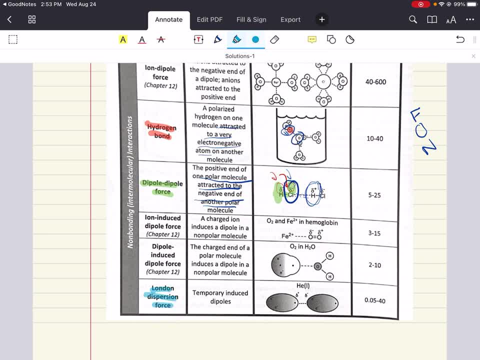 chapter: All right, London dispersion forces. What is it that holds nonpolar substances together in the solid or liquid state? It is this force, the London dispersion force, All nonpolar substances we know. it does not possess a permanent dipole with a positive and 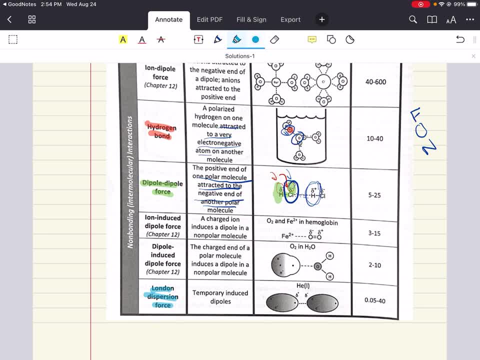 negative charge, All right. contrary to polar substances, which do Well with nonpolar substances, can they still form intermolecular attractions with other molecules? Well, of course, the intermolecular forces that hold nonpolar molecules together are the ones that are called 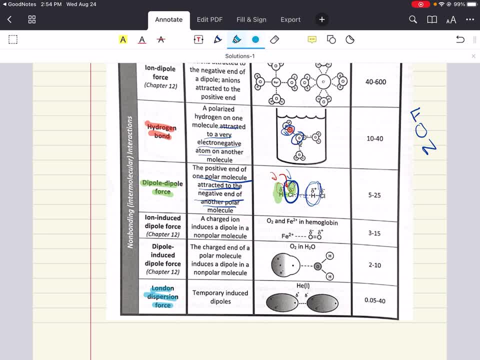 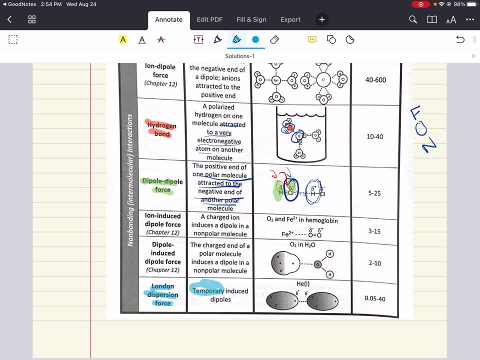 London dispersion forces, And these are attractive forces That are due to temporary- All right, this is very important- Temporary induced dipoles, not permanent dipoles like polar molecules, All right. so that's very important to understand. London dispersion forces are temporary induced dipoles, All right. all molecules that interact. 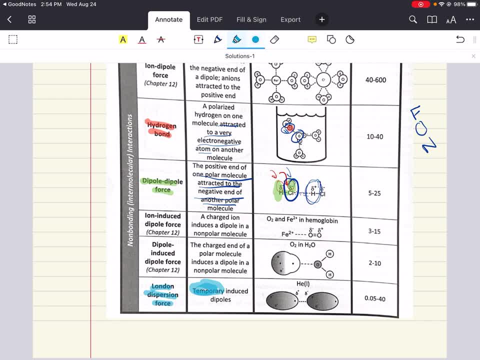 with other molecules. experience London dispersion forces period. All right, but it also explains the intermolecular attractions between nonpolar Molecules as well. All right. Now for the new intermolecular forces for this chapter that we have not covered before. the first one we're going to cover is ion dipole force. All right, Many. 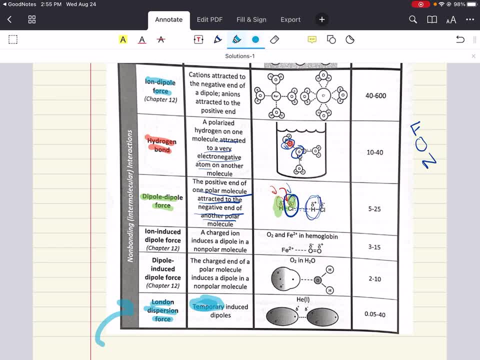 ionic compounds are going to be so soluble in polar substances like water, The positive or negative end of polar molecules is going to be electrostatically attracted to an ion of opposite charge. So when I compounds dissolve in water they're going to break into their cations and they're going to 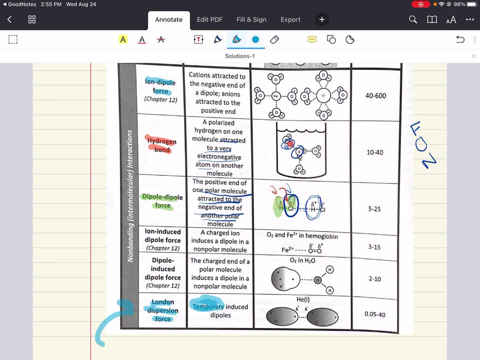 break into their anions, Those cations and those anions. they're going to interact with the polar solvent, the polar molecule. They're going to be electrostatically attracted to that with their opposite forces. This is called ion-dipole force Cations attracted to the 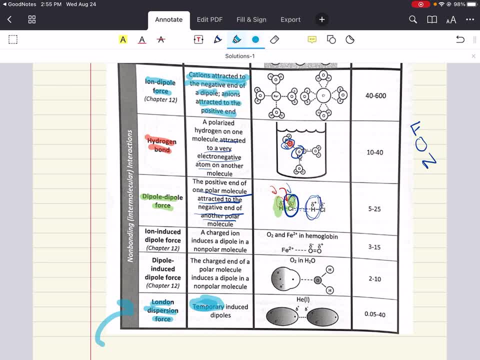 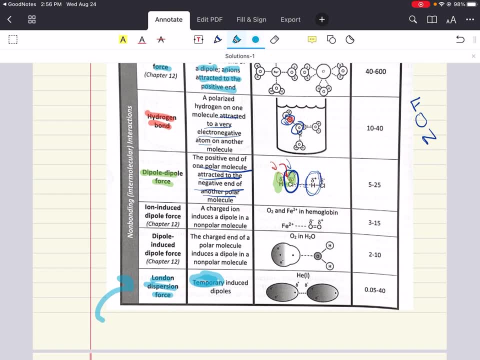 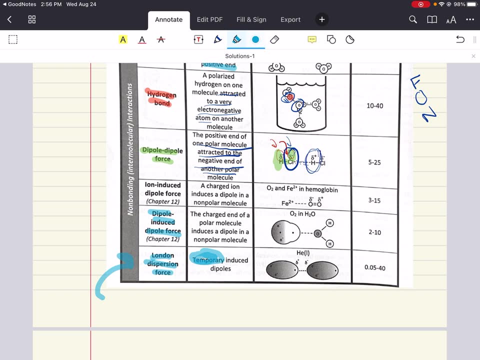 negative ends of a dipole and ions attracted to the positive ends of dipoles. Fantastic, That is ion-dipole force. The other one we want to cover is dipole-induced dipole force or attraction When a non-polar substance like water- I'm sorry, not like water, oh my God- When a non-polar 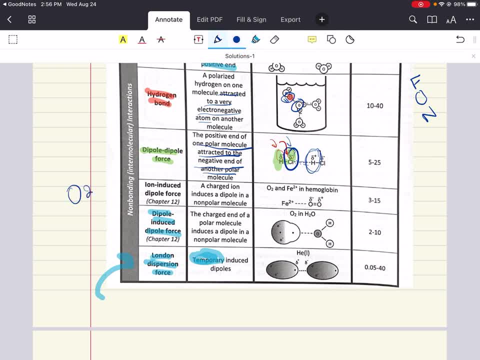 substance like oxygen, all right. like O2,, all right. dissolves in a polar solvent, all right. when we dissolve it in a polar solvent. what happens? Well, when we dissolve it in a polar solvent, the molecules are going to experience. 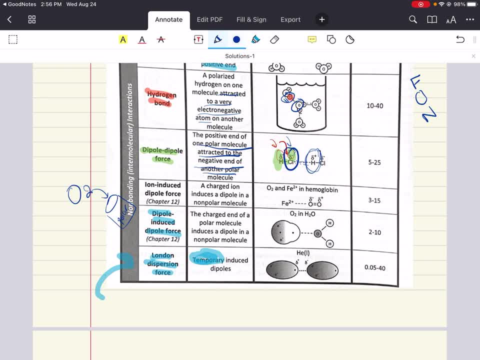 an intermolecular force that's going to be referred to as a dipole-induced dipole attraction. right, We have this non-polar molecule within a polar solvent or within a polar solvent, All right. What is it going to experience? This non-polar-polar interaction is going to be called. 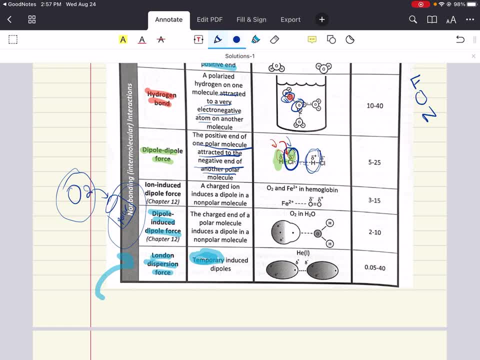 a dipole-induced dipole attraction. The charged end of a polar molecule- all right, is going to induce a dipole in the non-polar molecule, All right, And so that's why it's called a dipole induces a dipole for the non-polar molecule, All right. So that's one way of thinking about it. 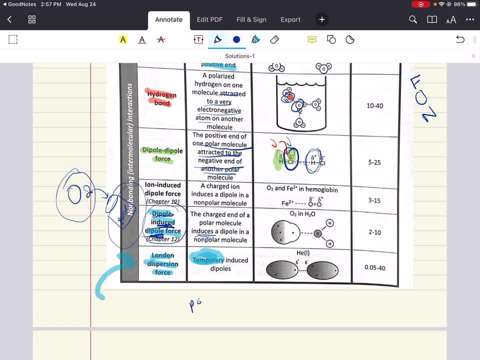 All right, A dipole-induced dipole. Dipole force happens between a polar and non-polar molecule. All right, This polar molecule has a dipole. right, We've talked about how polar molecules have this permanent dipole moment. This polar molecule with a dipole moment is going to induce a dipole moment. 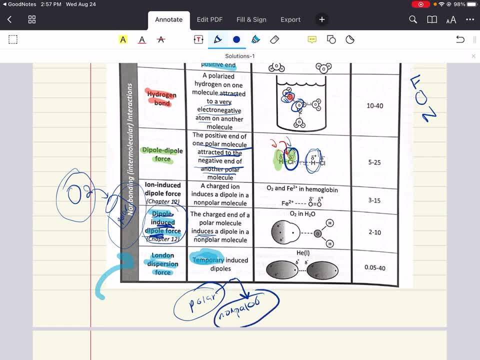 a temporary one in the non-polar molecule. All right, And so now we have a dipole-induced dipole force. Once again, the charged end of a polar molecule induces a dipole In the non-polar molecule. Fantastic, And last but not least, ion-induced dipole attractions. 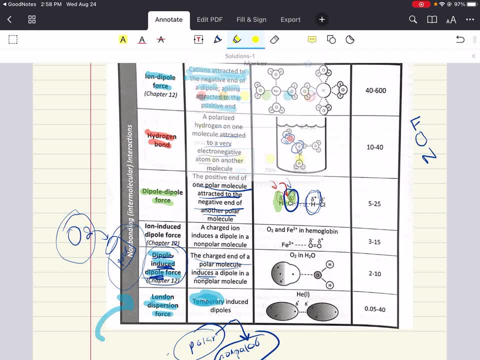 All right. Here let's highlight it in a new color Here. a charged ion- all right- is going to induce a dipole in a non-polar molecule- All right. So in dipole-induced dipole we have polar and non-polar. In ion-induced dipole we have an ion and a non-polar. 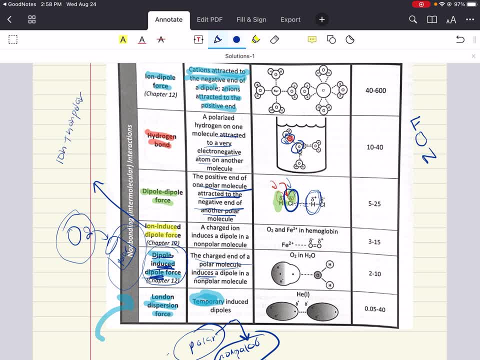 All right, So now you understand the distinction between these. All right. In an ion-induced dipole, a charged ion is going to induce a dipole in a non-polar molecule. The best example of this type of intermolecular force is the attraction between, say, a molecule of oxygen and iron. 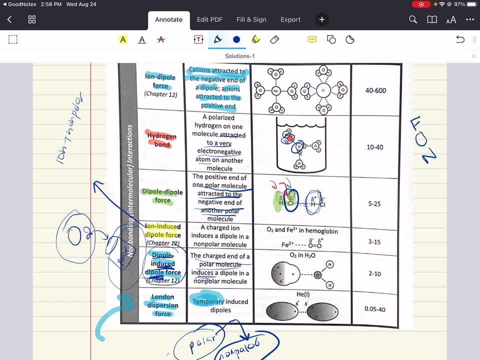 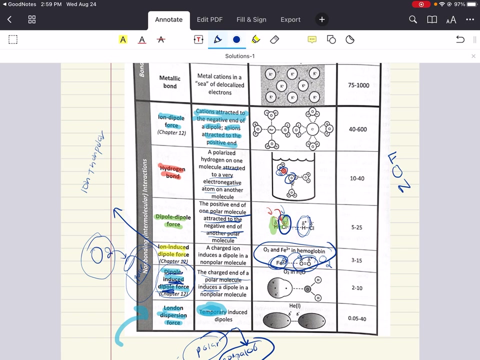 ion at the center of a heme unit and hemoglobin, All right. So that's a great example, right here. All right, The iron is an ion, All right, It has that two-plus charge. It's going to induce a dipole in this non-polar O2 molecule, All right. So these are our six intermolecular forces. 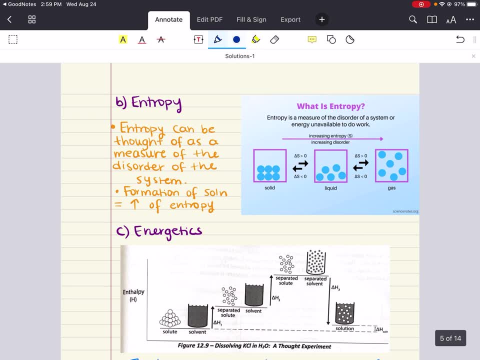 Fantastic. Now, that is one of the three factors that we wanted to discuss in order to understand the driving force in the formation of a solution. We're going to keep this brief and short, because we actually have a chapter coming up where we really dive into entropy. All right, What we're going to say now is that entropy can be thought. 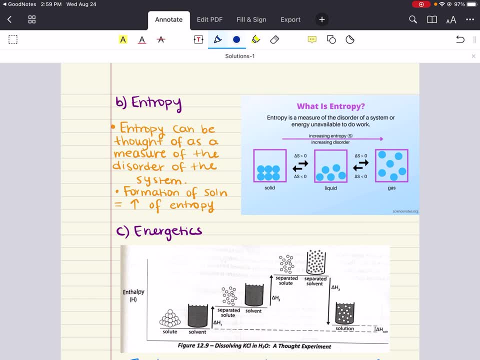 of as a measure of the disorder of the system. This is not a complete definition of entropy by any means. All right, This is something that needs to be understood. This is the best sort of definition. with our current understanding of chemistry, Entropy can be really dived into. 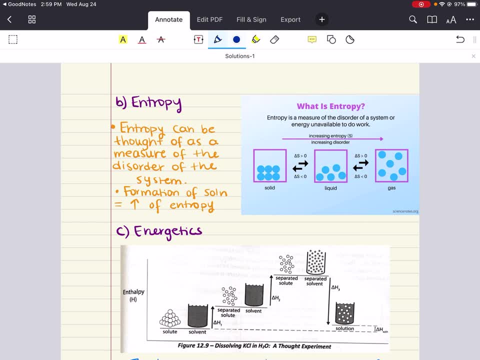 a better definition, a more mathematical one, but that's really for physical chemistry. So if you're interested in that, you should check out my physical chemistry playlist. that's currently being developed, But for now, this is good for now, for this chapter. 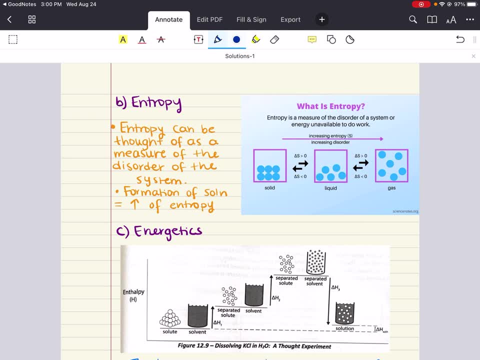 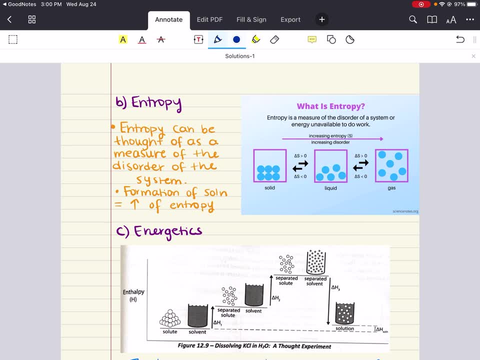 randomness and disorder. Nature likes that. The formation of a solution is actually usually accompanied- guess what- by an increase in the entropy of the system. All right, The third thing we want to cover in order to understand the driving force of formation of solutions is: 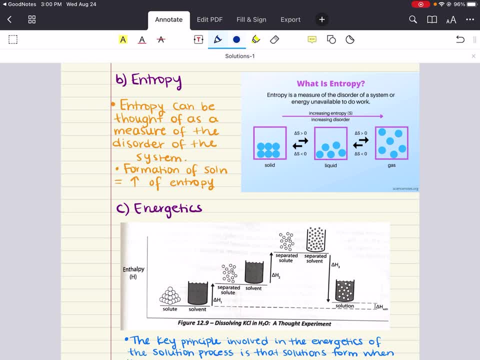 energetics of the solution process. So in general chemistry one, we learned that bond breaking is considered endothermic, Bond formation is considered exothermic. This principle, which is guess what? it also applies to intermolecular forces and attractions. So two molecules that. 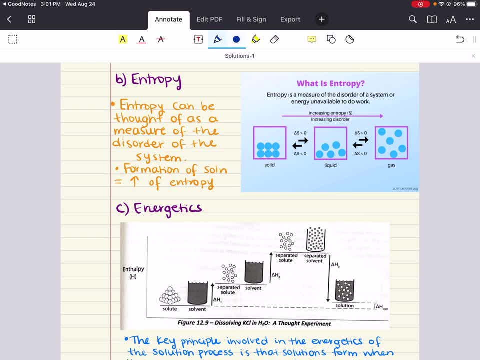 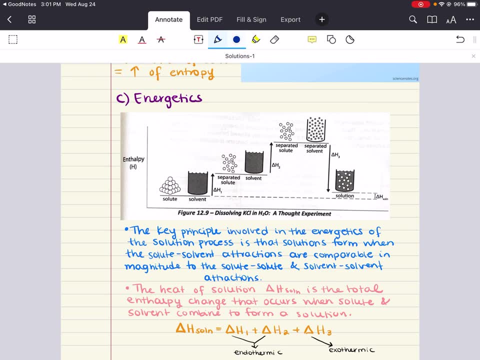 are going to be held closely to one another by intermolecular attractions are going to have a lower potential energy than when they are separated. Therefore it's going to require energy to pull molecules apart and overcome that intermolecular attraction in an endothermic. 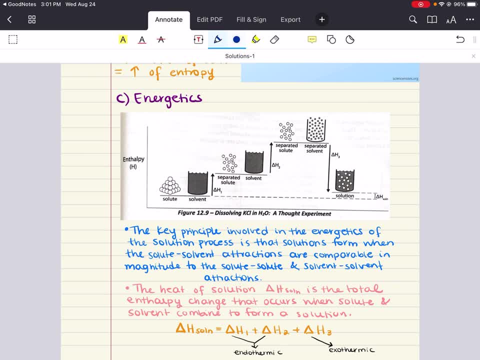 process. Conversely, on the other hand, when separated molecules come together as a result of intermolecular attractions, their potential energy is lowered and energy is actually released. All right, So then we can say that the coming together of solute and solvent particles is then. 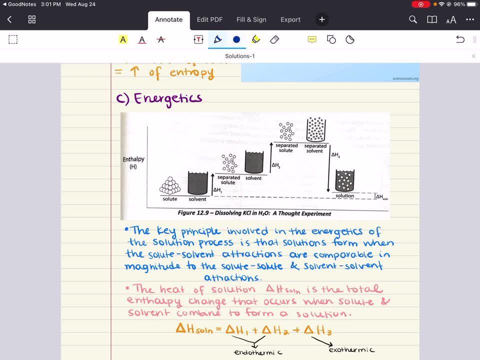 an exothermic process, All right. And the energetics of the solution process can be actually summarized in terms of this Key principle: solutions form when the solute solvent attractions are comparable in magnitude to the solute solute and the solvant solvent attractions. All right, This sentence is important. 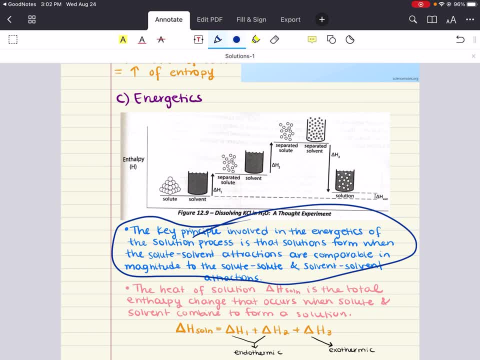 for you to understand, All right Solutions form when the solute solvent attractions are comparable in magnitude to the solute solute solvent solvent attractions. another way of saying this is that in order for a solution to form the energy that is required to separate solute particles and solvent particles. 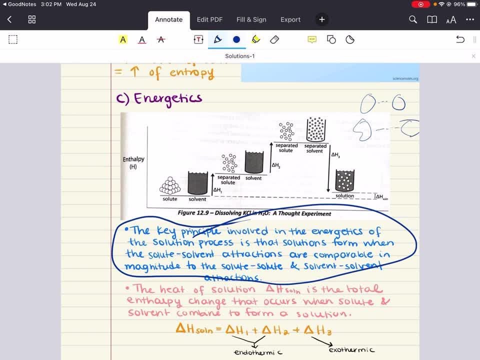 all right, must be compensated by the energy released when the solute and solvent particles mix. all right, so let's actually really consider this by looking at this diagram. all right, this is a good thought experiment. all right, we have potassium chloride in water. the solution process can be imagined to occur in three important steps. all right, three important steps. the first stage: 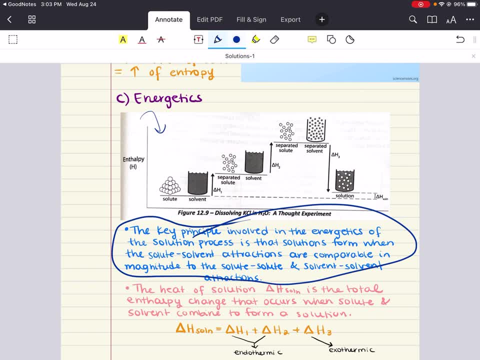 involves overcoming the solute solute attractions. all right, in this imaginary step, the ionic bonds holding the ions together in potassium chloride have to be broken in order to allow the separate ions to go into solution. so this first step is solute solute attractions must be overcome. all right, solute, solute. actually, i can't. 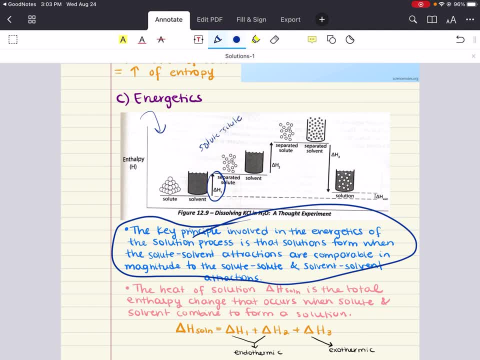 solute. solute attractions have to be overcome, step one. so your potassium chloride has to be really separated into just potassium and just chloride. all right, that's our first step, fantastic. in the second stage, the solvent- solvent attractions must be overcome in order to make room for the solute. all right, so in this, 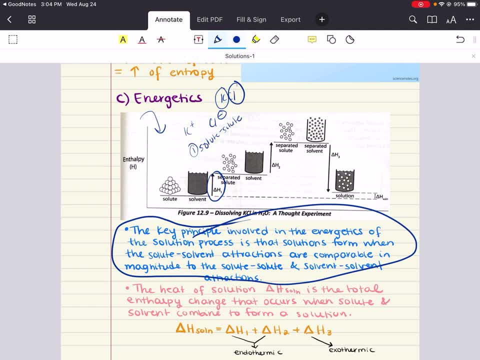 example, the. the water molecules are going to be held together by hydrogen bonds. so we have to overcome those hydrogen bonds in water. so we have to overcome those hydrogen bonds in water, all right. as the second step, to overcome solvent solvent attractions, all right. so first overcome solute solute attractions, next we have to overcome solvent solvent attractions. so now we have. 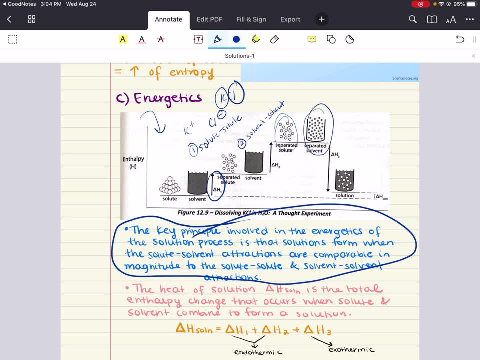 separated solute, we have separated solvent, they can finally really, you know, begin to form a solution. all right, so now, overcoming the hydrogen bonds in water, we can move into the solution. so the third stage: solute solvent attractions are formed. All right, The coming together of solute. 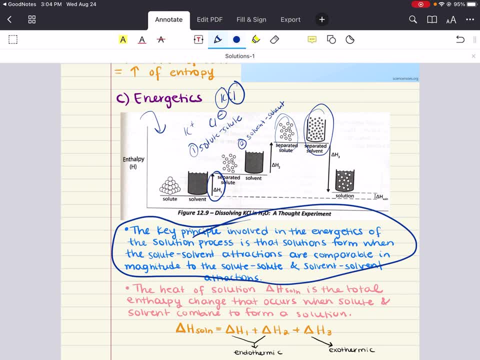 and solvent particles. All right, Is that last, final step? So first we had to overcome solute solute attractions. All right, This required energy, So it's endothermic. overcoming solvent solvent attractions also required energy. right, Cause you're breaking. you're breaking. 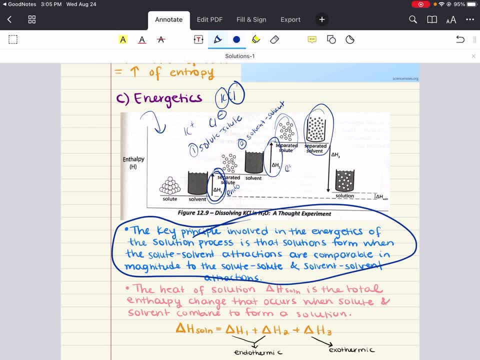 intermolecular attractions in both of these. All right, So they require energy. They're endothermic. Then, finally, when you have the solute and solvent separated, they can begin to form a solution. Forming a solution is an exothermic process, So it releases energy and 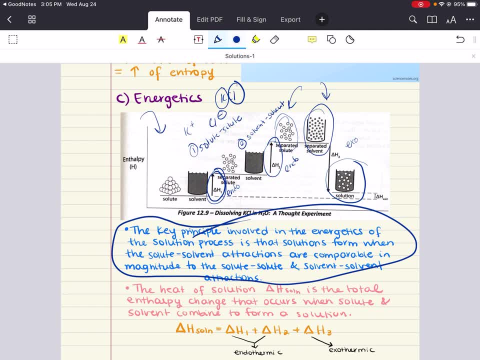 voila, you have reached solution. All right. Now the clustering of solvent molecules around a solute particle is the third stage that we talked about here. when we're forming a solution, And this is called solute. We've talked about this. The solvent is going to start to cluster around the solute. All right, 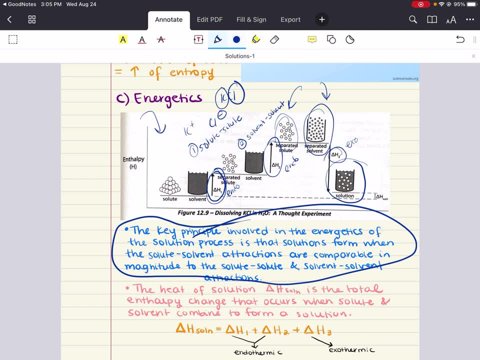 Now another term for this: Delta H3,. right, When the Delta H3, the, the, the enthalpy associated with making a solution. this solute solvent attraction has another name: It's called heat of hydration. All right, It's called heat of hydration. It represents the total enthalpy. 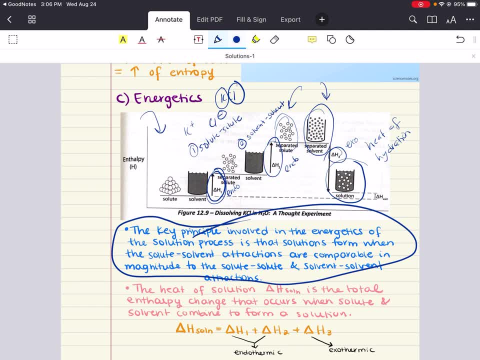 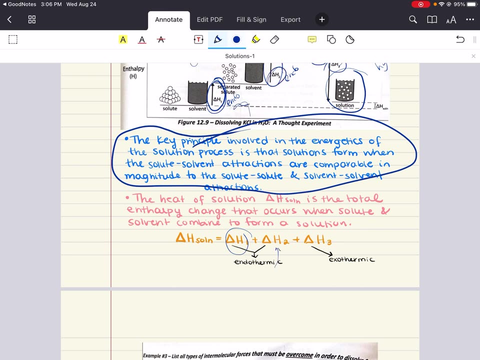 change um for forming a solution. So it's exothermic, since it lowers the potential energy of the solute and solvent particles. Now, the sum of all of these three steps, all right, the sum of Delta H1,, the sum of Delta H2, the sum of Delta H3, all together, the sum of this is called heat. 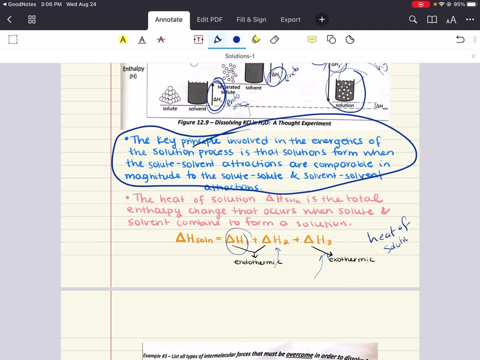 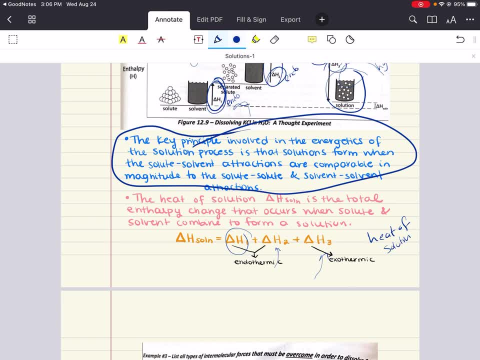 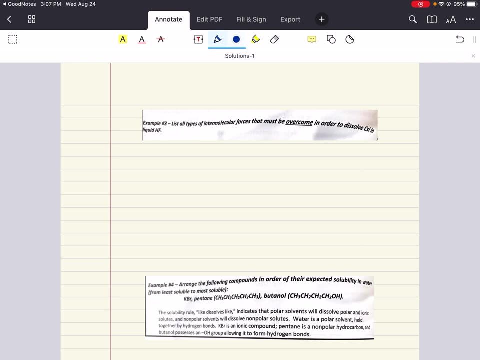 when solute and solvent combine to form a solution. All right, So there it is, the energetics of the solution process. Perfect, Now let's do some practice problems. All right, This practice problem says lists: list all types of intermolecular forces that must be overcome in order. 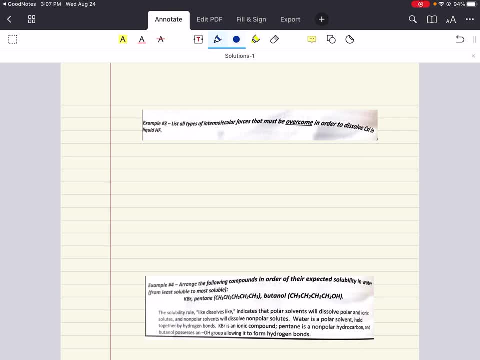 to dissolve CCM iodide in liquid hydrogen Fluoride. All right, We need to list all the intermolecular forces that must be overcome in order to dissolve- to dissolve these things in each other. Notice that this question is not asking about the intermolecular forces that are formed between the solute and solvent. 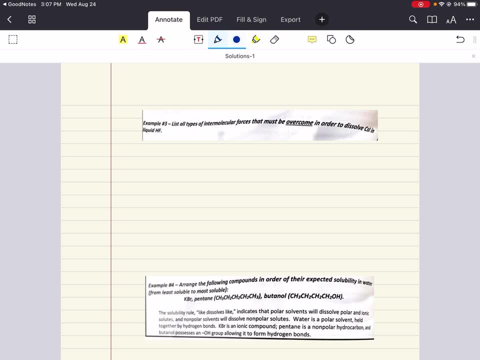 No, it's asking you what? what intermolecular forces need to be overcome in order to form a solution. So what it's talking about is the solute- solute and the solvent- solvent forces that must be overcome in order for the solution to form. So we're going to look at each one of 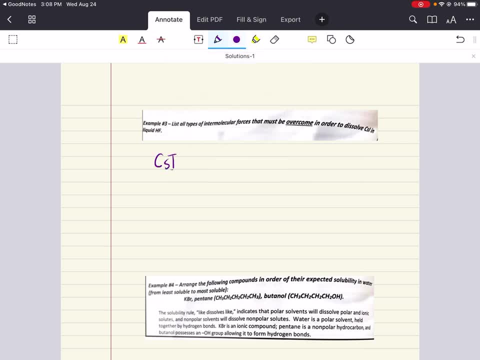 these molecules independently. All right, The first one: All right. The solute: This is an ionic compound. All right, This is an ionic compound. Perfect, We know this, because this is metal, non-metal, All right. 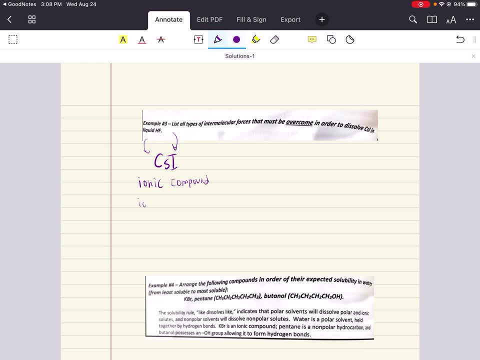 Its particles are going to be held together by ion, ion force, All right, Or ionic bonds, because this is an ionic compound Now in the liquid hydrogen fluoride, All right, The separate molecules are held together close to one another by hydrogen bonds, All right. So 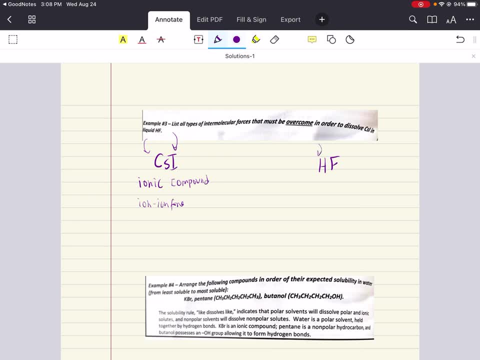 the polarized hydrogen in one molecule of hydrogen fluoride interacts with the fluorine of another hydrogen fluoride. All right, So what does that mean? What that means is that we need to overcome ion, ion forces, and we need to overcome hydrogen bonds as well, Something else that needs to be overcome. 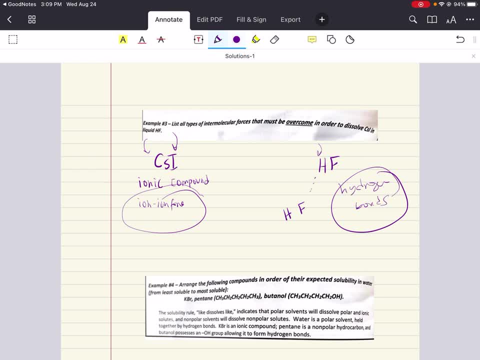 Sometimes people forget about this, but remember, in in all molecules that are interacting with other molecules, London dispersion forces also exist. All right, London dispersion forces also exist. So the intermolecular force that needs to be overcome for CCM iodide. 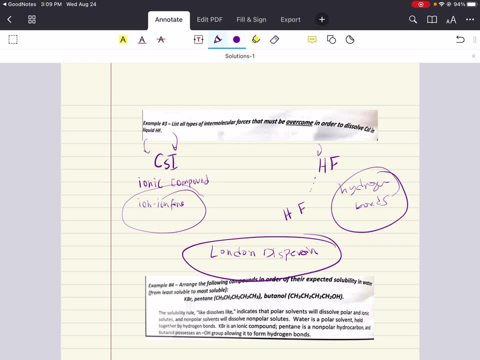 has to be ion ion force- right, Because this is an ionic compound and ions are going to interact with other ions dissolved in solution- Fantastic. We also have to overcome hydrogen bonds- All right, because we're going to have hydrogen fluoride and the hydrogen of one. 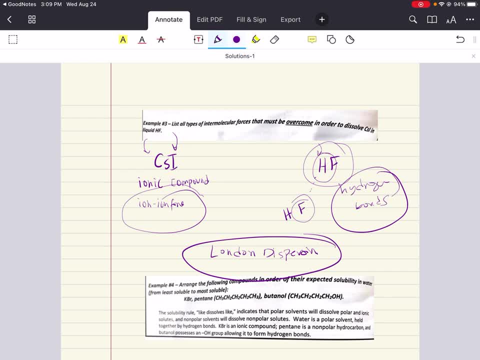 hydrogen fluoride is going to interact with the fluoride uh of another hydrogen fluoride molecule And of course, these both have London dispersion, All right. So we're going to have hydrogen fluoride and the hydrogen of one hydrogen fluoride is going to interact with the fluoride. 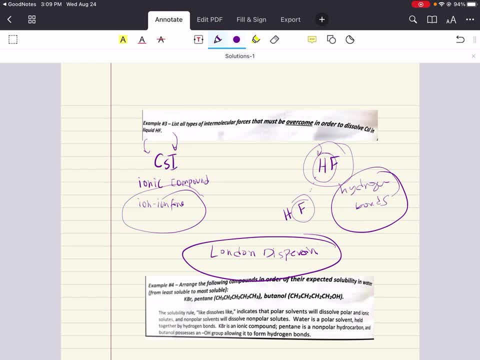 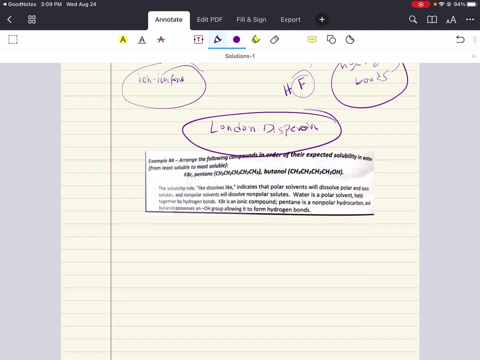 All right, So we're going to have hydrogen fluoride, and the hydrogen of one hydrogen fluoride is going to interact with the fluoride, And so those are the three intermolecular forces that need to be overcome to form a solution. Fantastic. Now this problem says: arrange the following compounds in: 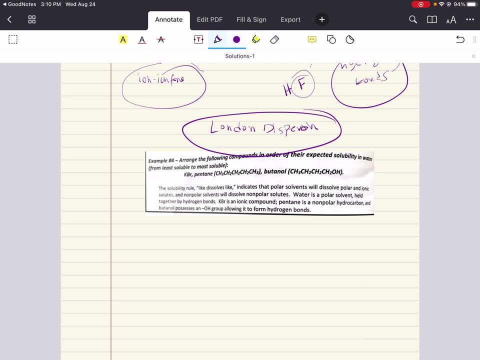 order of their expected solubility in water, So going from least soluble to most soluble. If you remember the solubility rule, like dissolve likes, which means that polar solvents are going to dissolve polar and ionic solutes and nonpolar solvents are going to dissolve nonpolar. 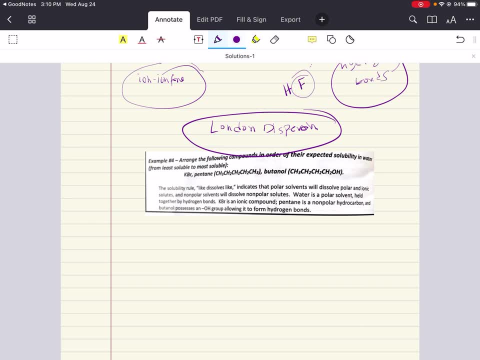 Solutes water. water is a polar solvent, All right. Water is a polar solvent. It's held together by hydrogen bonds, All right. So we have to keep in mind that hydra, that that water is polar, All right, When we look and investigate each one of these molecules that were given. 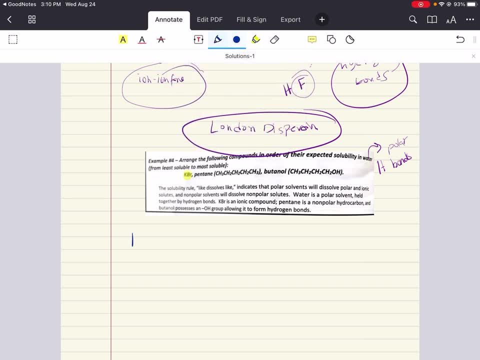 now KBR. KBR is actually an ionic compound. All right, This is an ionic compound. This is an ionic compound, All right. Pentane- pentane is a five carbon hydrocarbon chain. All right, It looks like this: five carbons attached to each other: One, two, three, four, five, with. 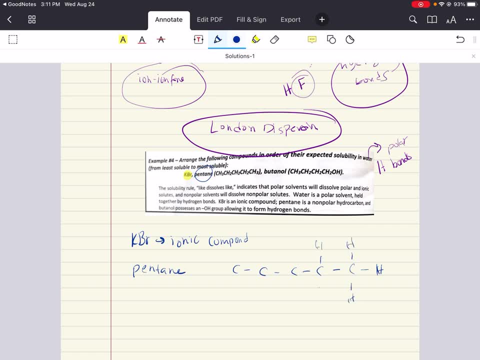 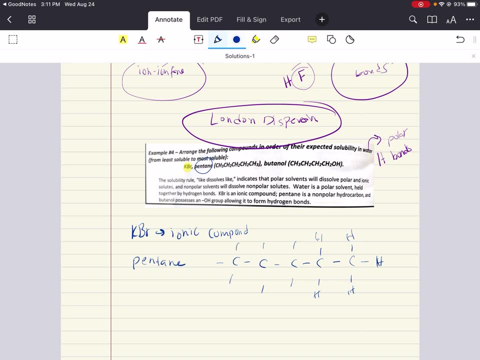 a bunch of hydrogens, All right. Lots and lots of hydrogens, All right. That's pentane. I'm not going to draw all the hydrogens, but all those blank spots- spots would be hydrogens. Pentane is actually a nonpolar. 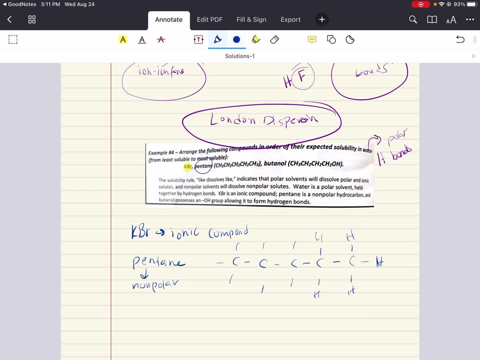 Molecule. It's just a hydrocarbon where there's no polar bonds whatsoever, So it's a nonpolar molecule. Butanol- butanol is four carbons attached to each other, a four carbon chain with an alcohol group. So butanol looks like this. We're going to draw it out: Butanol. 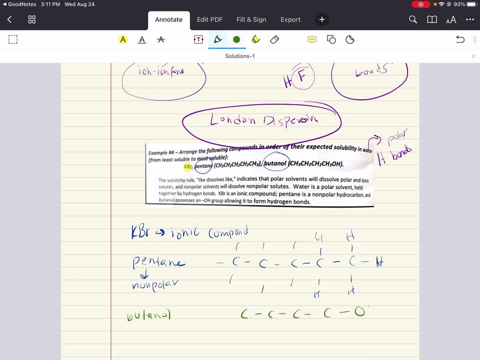 All right, We have four carbons and an alcohol group. all these empty bonds that I'm drawing Our hydrogens. OK, Butanol is a polar molecule. All right, It possesses an alcohol group that's going to allow for potential hydrogen bonds. All right, Awesome, Fantastic, All right, This is 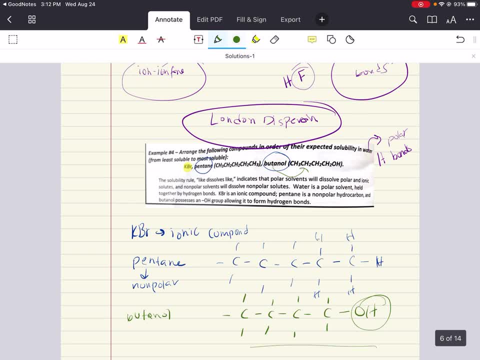 butanol right here, just in molecular form. I just wanted to draw it out. All right, So we have these four molecules: KBR, ionic, pentane, nonpolar, butanol, polar. Sorry, three, I guess. 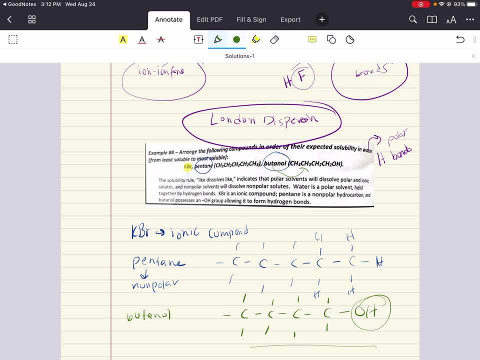 we count Anyways. So KBR is ionic, All right, It's going to be highly soluble in water. Pentane is non-polar, All right, Water is polar, Remember- like dissolves, like. so Pentane, which is nonpolar, is probably not going to dissolve in water, All right. And butanol: 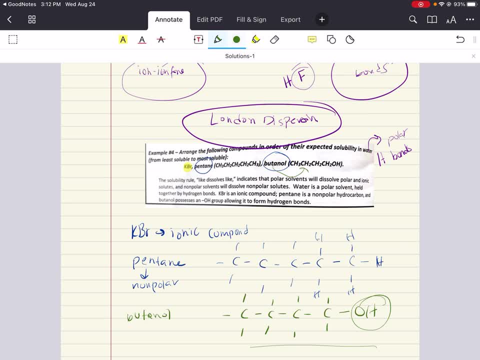 can form hydrogen bonds with water, So easy off the bat. Pentane is going to be a nonpolar hydrocarbon. It's going to be the least soluble. But is there a way to distinguish now between KBR and butanol? Which one is better, Which one is more?